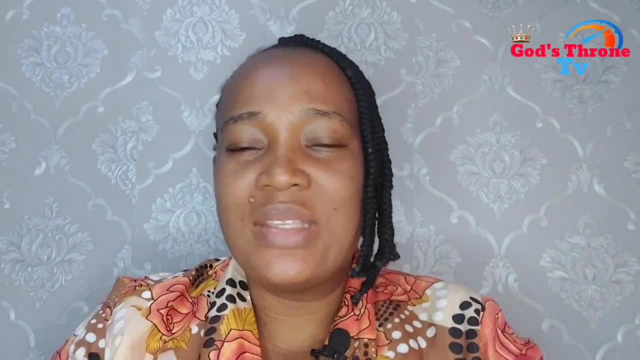 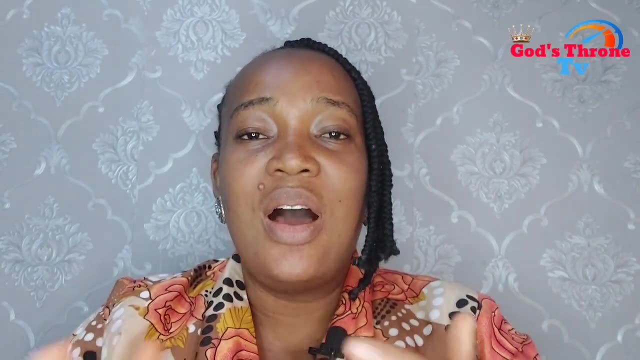 I upload videos every single day. Good week, Wednesday and Saturday. God bless you. and to all my subscribers I want to say thank you for coming back to watch my videos. All right now to this video. Now, what does it mean to see? 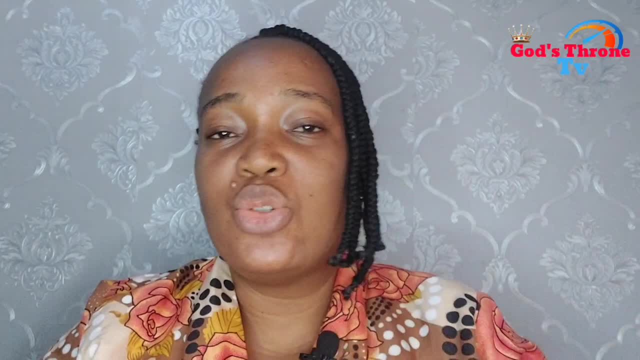 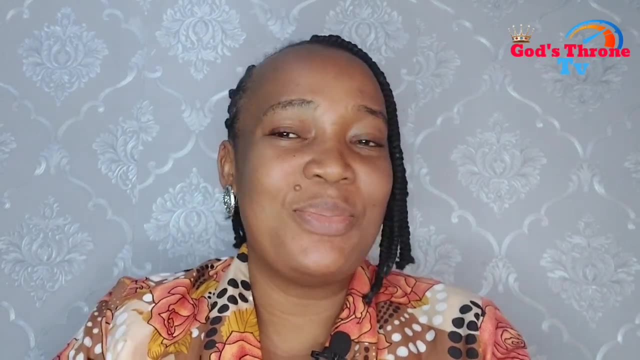 purple colors in the dream. So today I want to share with you, you know, open your eyes to the world of purple- okay, to the world of purple. So stay with me. I want you to understand that purple can also have, can have a positive meaning and also can have. 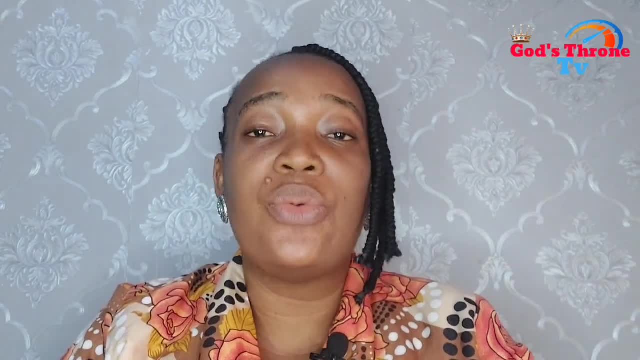 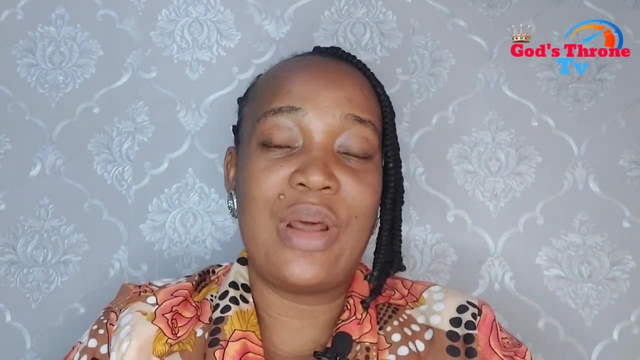 a negative meaning. So in this video today, I'm going to share with you, first of all, the positive meaning of purple colors. So generally purple color. if you see me look down, please just know that I'm. I wrote down some things. All right now, purple color generally. 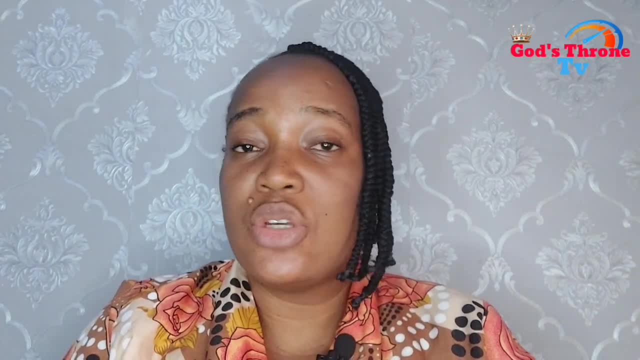 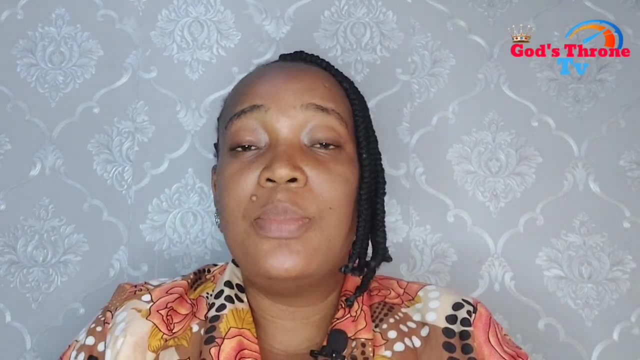 could mean, um, a supernatural, a spiritual authority. Okay, On this channel, I give you biblical and spiritual dream interpretation. Now, the Bible is also a gateway for our interpretation and whatever we do on this channel is given according to the Holy Spirit. So today I want to 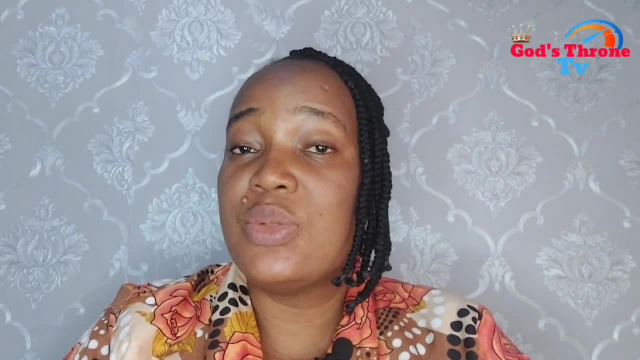 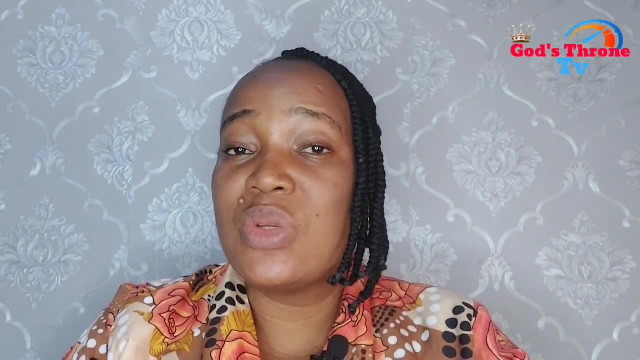 share with you. you know what I do on this channel is given according to the inspiration of the Holy Spirit. So whatever interpretation you get here is according to the inspiration of the Holy Spirit, And remember that what you know, the scripture, was written according to. 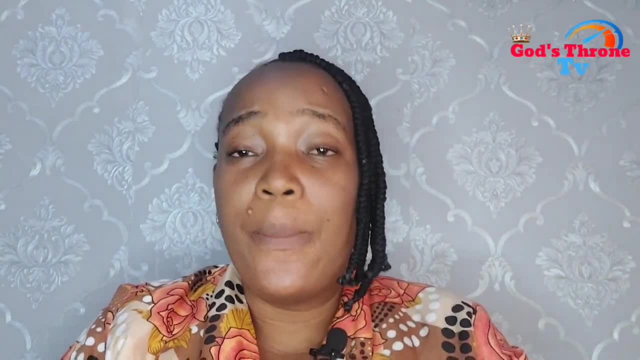 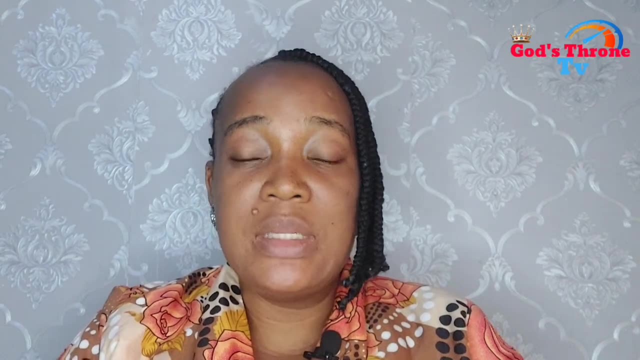 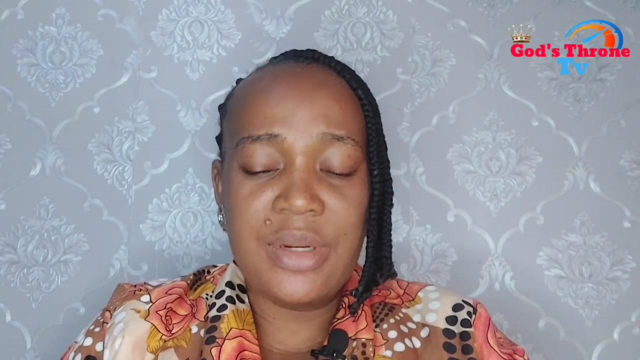 the inspiration of the Holy Spirit. So it was inspiration of God upon men that were able to make them write the scriptures. Oh, ordinarily purple means nobility, purple means royalty, purple means wealth, It means authority. Now there are many examples in the 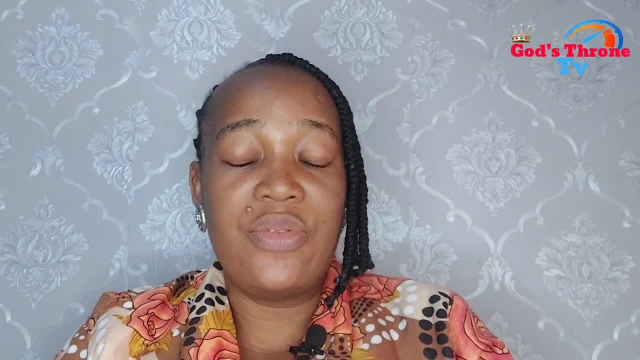 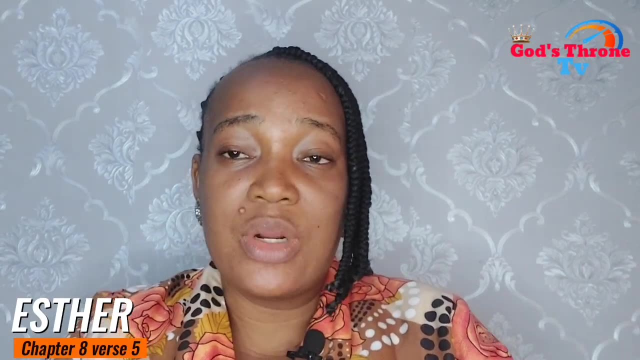 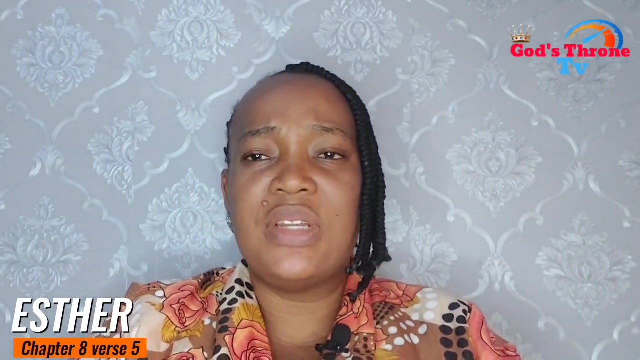 scriptures where we talk about purple. Now, in the book of Esther, chapter 8, verse 5, um in the um, talking about Mordecai, um going the presence of the king with a large crown and a garment of linen and purple, Okay. And the book of Daniel, chapter 5, verse 7, also um, you, you, you see. 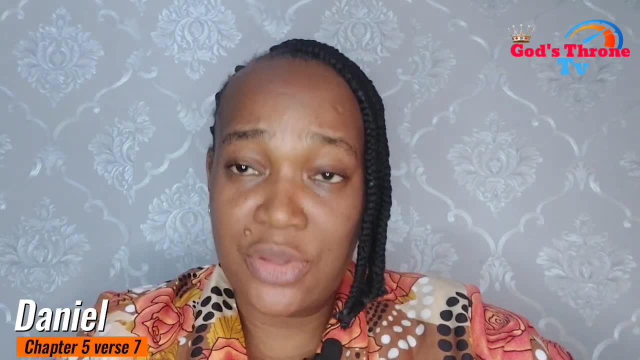 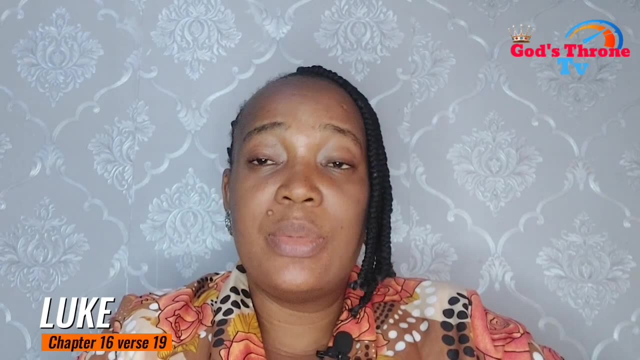 that, um, it's also a symbol of, of authority. there And in the book of um, Luke, chapter 16, verse 19,. um, it's talking about the rich man that dressed in a purple outfit or purple apparel. So when we talk, 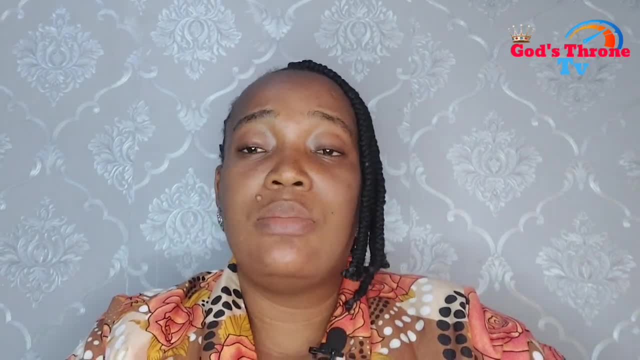 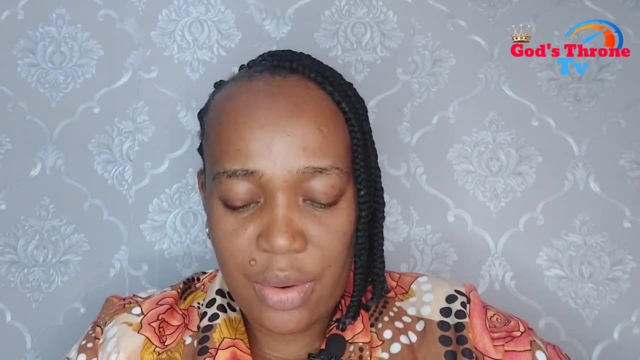 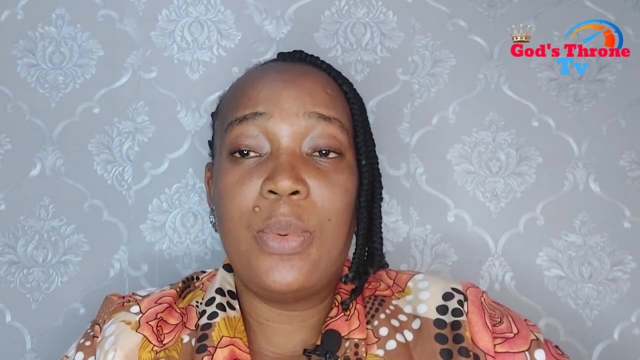 about purple generally mean. I've told you the meaning. it means nobility, It means um, um authority. It means um royalty, It means wealth. All right, Now let's talk about the positive meaning of purple. All right And um. like I said in the other time, purple means authority. 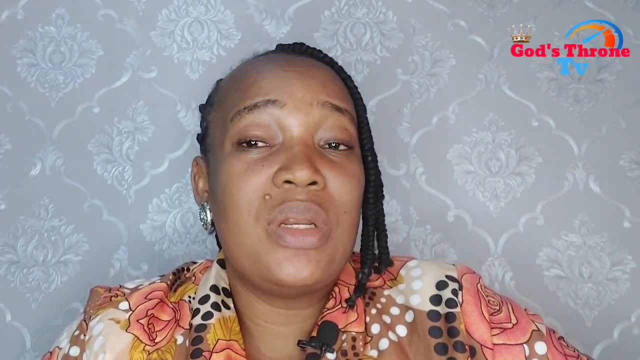 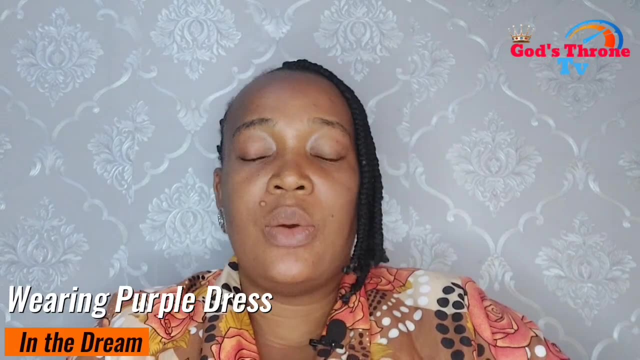 Now, when we look about them, when you see purple, you wearing a purple dress in the dream, it could mean um a spiritual authority. It means spiritual authority And I thought, when I say spiritual authority, I mean God giving authority. Okay, God has given. 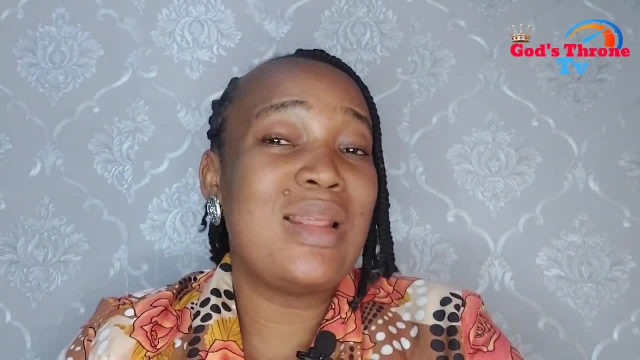 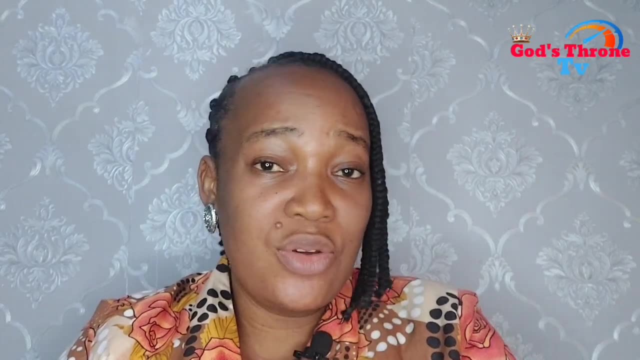 you this authority. It could also mean that what you are doing at that point in time, you are on the right path. Okay, You are doing what you're supposed to do, which means you're ruling in that aspect that you find yourself, which means you're, you are in charge with me. Um, you're making 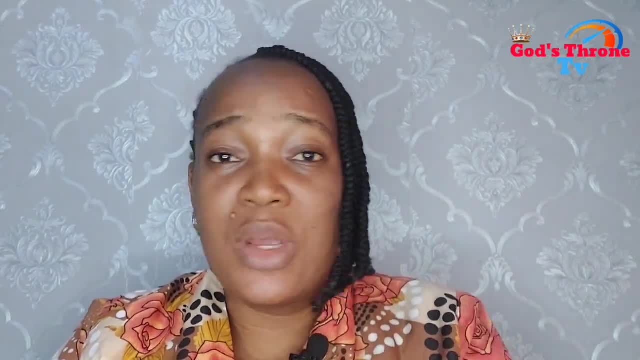 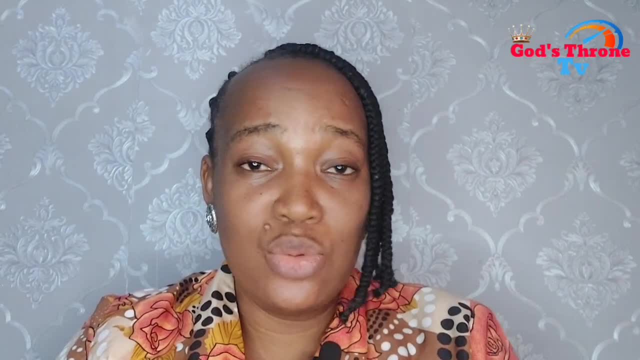 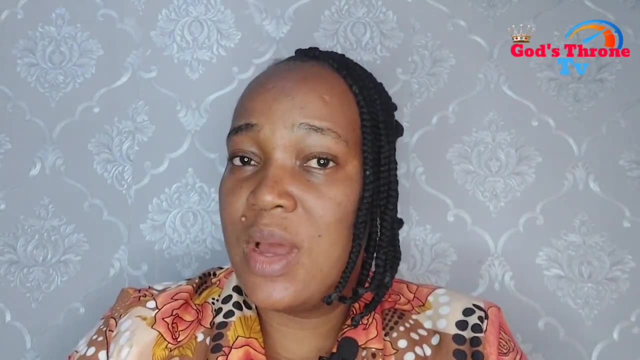 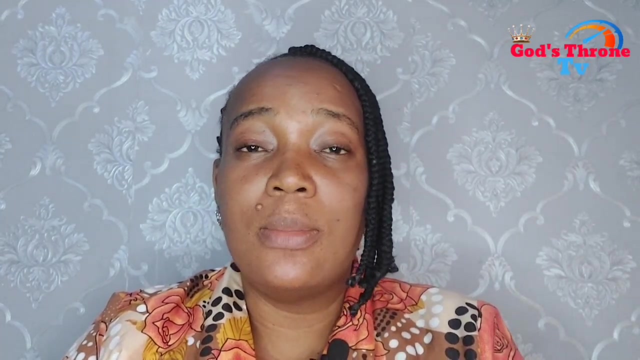 to destiny and identity. Yeah, Maybe don't know what authority means Authorities linked to identity. It means to destiny. Now, I said this just a while ago, that when you see yourself wearing a purple dress, it means that, um you are, you are in charge, or um, um, you are ruling. Okay. 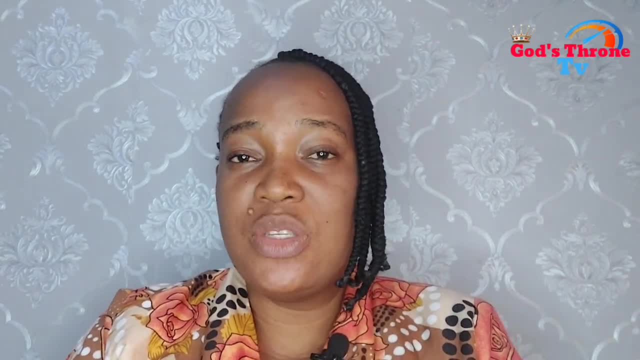 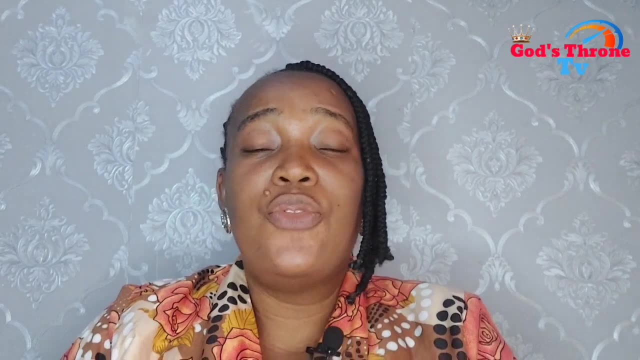 And when I said authority and destiny, which means you are in the right path of your destiny, now there is um. it's a very great error in a man's life for him to walk in the opposite of his destiny. it's a there's a big error for someone to walk in the opposite direction of 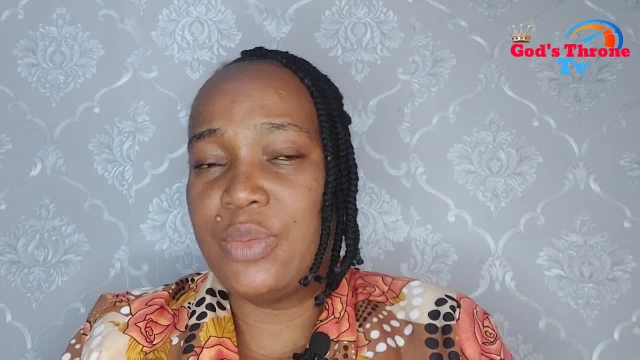 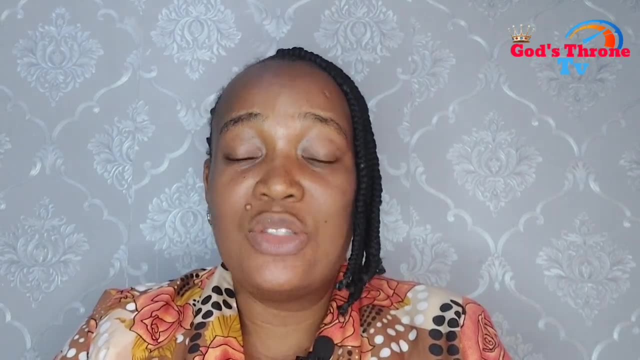 his destiny. yes, that's the truth. so, but when you see yourself wearing a purple dress in the dream is trying to tell you spiritual authority, and authority means your destiny and your identity, which means you are fulfilling god's given destiny. you are on the right path, you have discovered your. 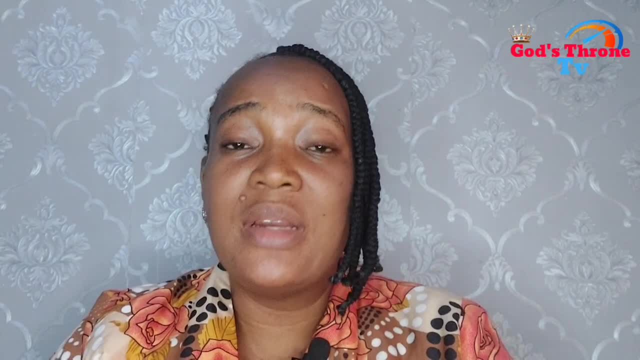 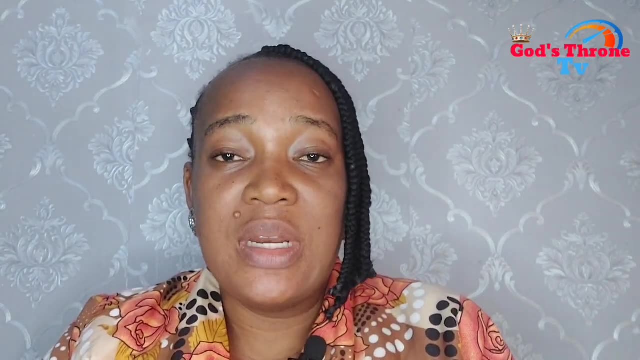 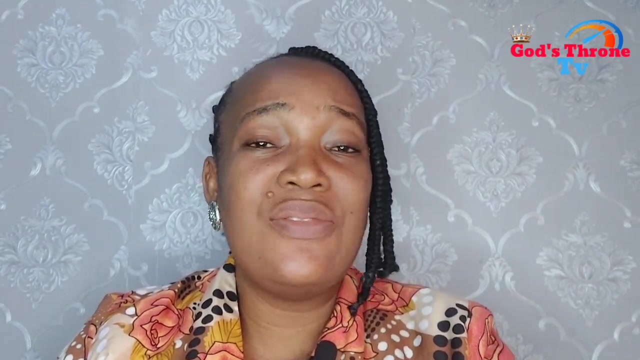 identity. okay, that you know who you are, all right. you know um the path you're supposed to go in life. i hope you get that now. oh, each of us have different rules in life. okay, each of us has, um what god has called us to do, and i want you to understand that god has created us in a very 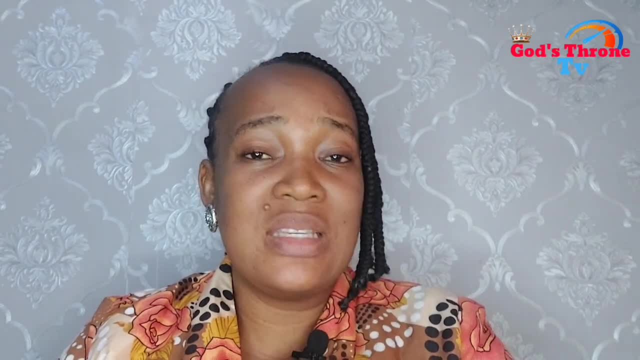 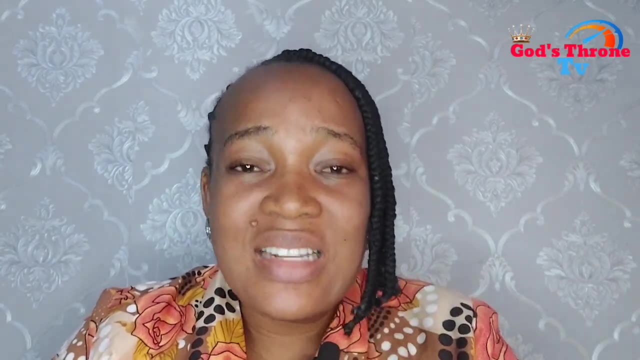 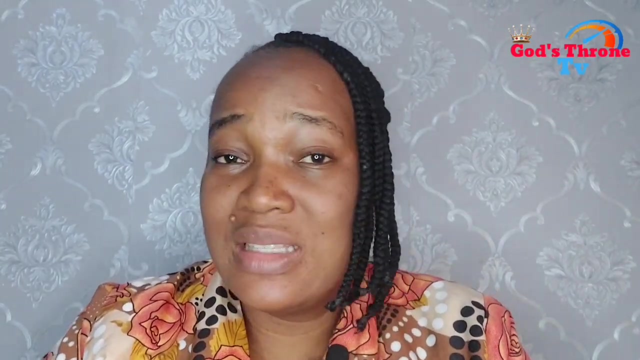 unique and beautiful way. what god gave me as a gift is different from what god has given you. that you're watching me as a gift now, it's not meant for you. it's not left for you to identify or discover what god has given you, or to be able to know the kind of gifts, to be able to walk in the destiny god's given. 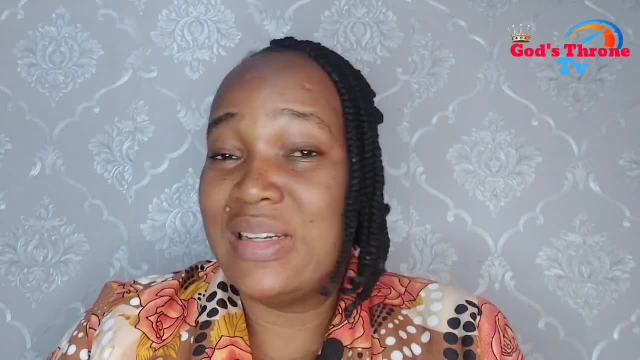 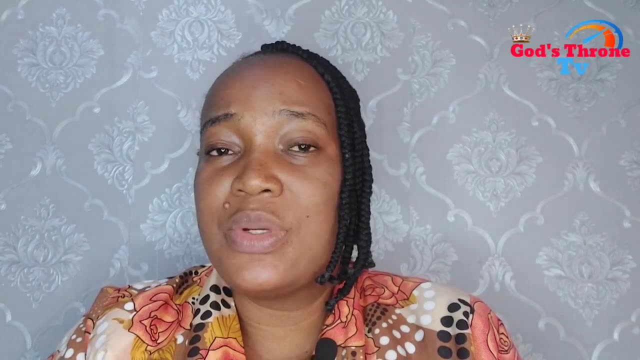 destiny or knowing your identity. because if you know all this- i'm just if you know all this- competition will be reduced. you will not want to compete with another person. so that is why when you see yourself in a purple dress in the dream, which means you know what you're supposed to do, 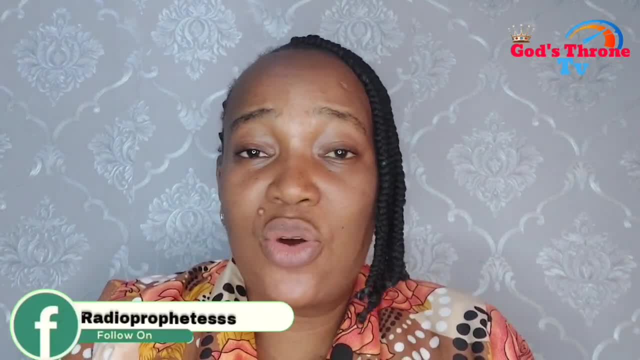 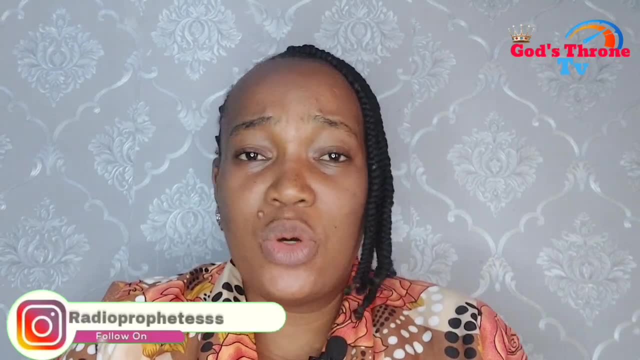 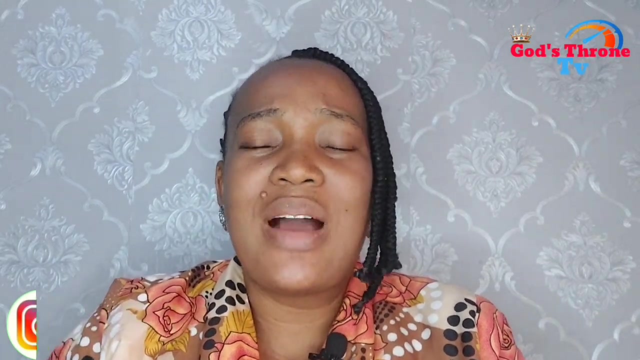 you are on the road on. you're on the path of discovery of out or of identity discovery. you are on the path of destiny discovery and i pray for you. is anyone watching me right now, when you find it very difficult to identify your person, to know who you are, you know? i pray that god will open your. 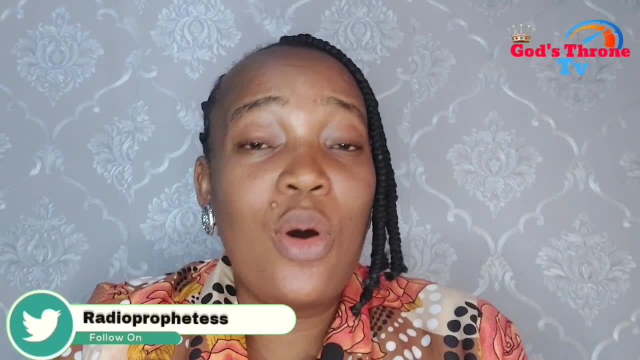 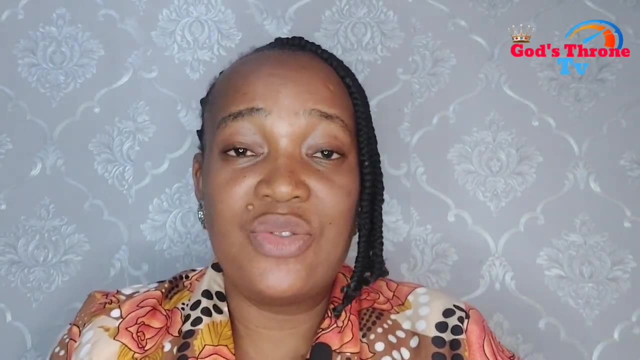 eyes, so that you will see and know the path that god really wants you to go, in the name of jesus. another thing: you must understand this dream. we feel that, ah, anybody can have this dream. i want to tell you that authority comes from god. yes, authority comes from god. and who? how can we get? 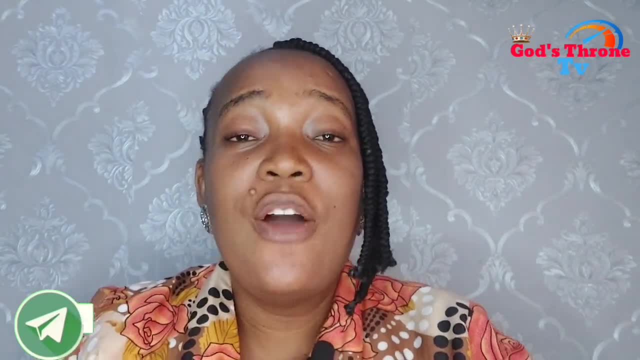 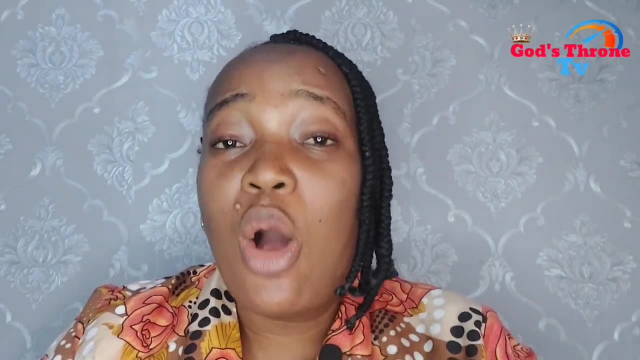 to this god, it is true, jesus christ. jesus christ is the only one who can have this dream, and i want to share that with you, because this is the only gateway to this planet. this is the only way to have that authority. okay, so the authority, and discovering your identity, discovering who you are comes from. 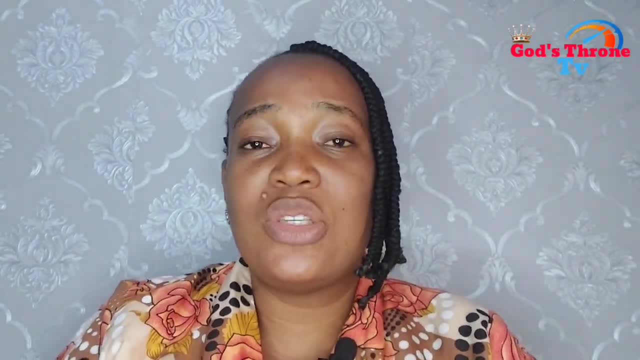 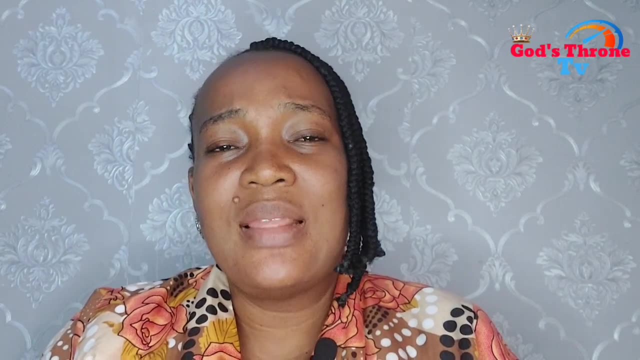 knowing god, your close relationship with god. i hope you are getting what i'm trying to say. so we are talking about purple, purple generally. now this kind of dream also come. it come to people that have um, that are. they are growing, there are matured. you know, when i said there, 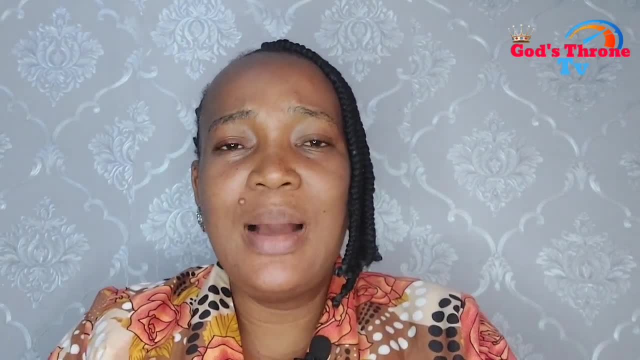 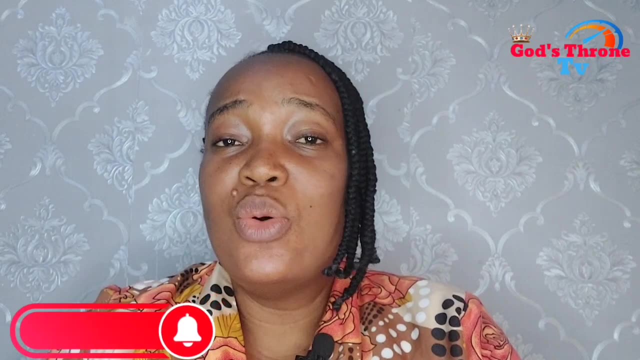 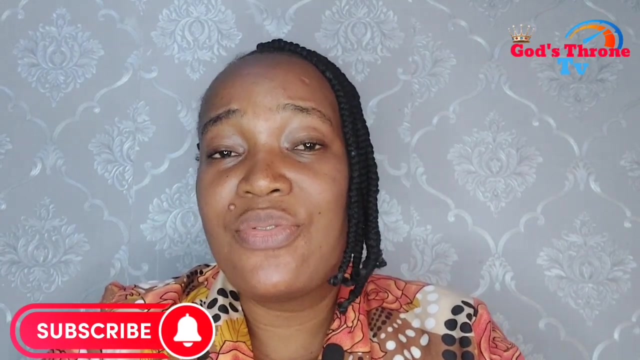 was a time i had this dream, some time ago, i think. the time i had this dream was um five, seven years ago, i think seven years ago- and um, when the dream came, i, the holy spirit, had, you know, dropped a lot of things in my mind. okay, so i i knew that god was preparing me for a 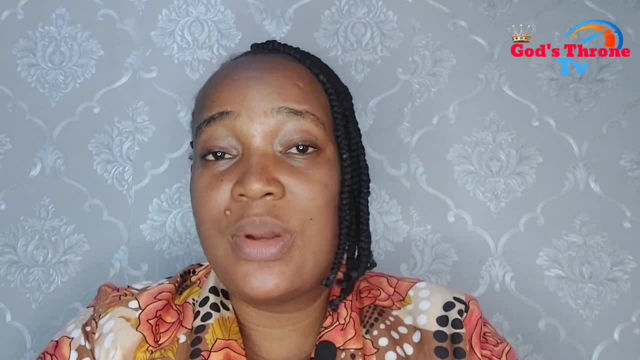 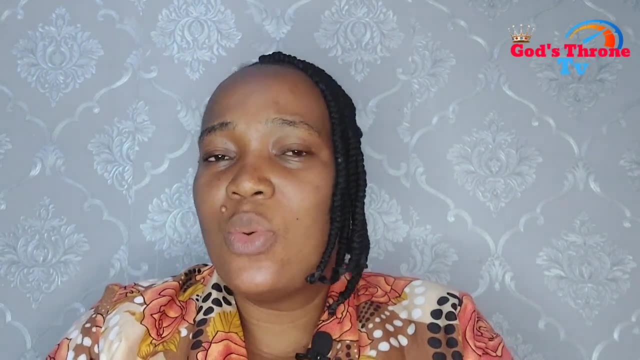 particular office. god was preparing me for a particular ministry, so when it came, i just smiled. i know that god i am, i god is leading me on the right path. so if you're watching me right now and you have had this dream- anything purple, purple dress- or you know you're wearing purple. 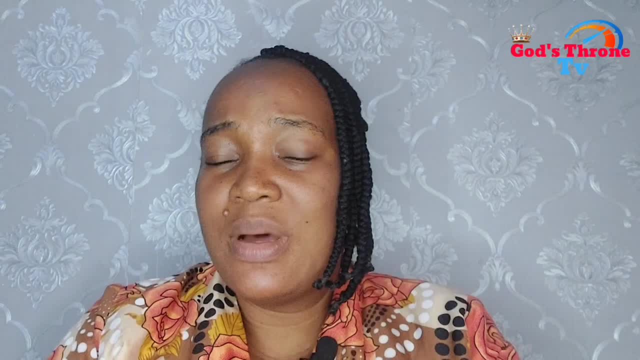 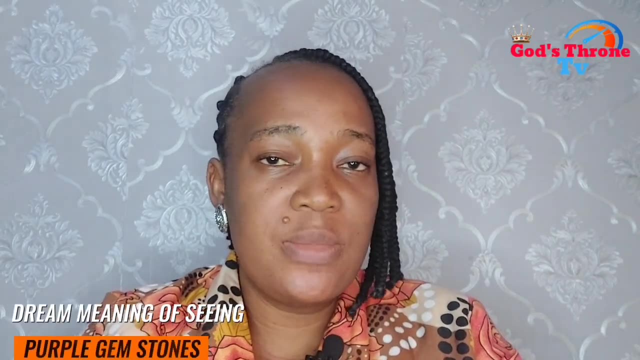 dress. you know. it means that, um, you are on the right path. it means that god is. god is opening your eyes to what you're supposed to do. that thing is that when you see purple gemstones- okay, purple gemstones, i hope you know what gemstones are now- this could also mean that, yeah, i've well. 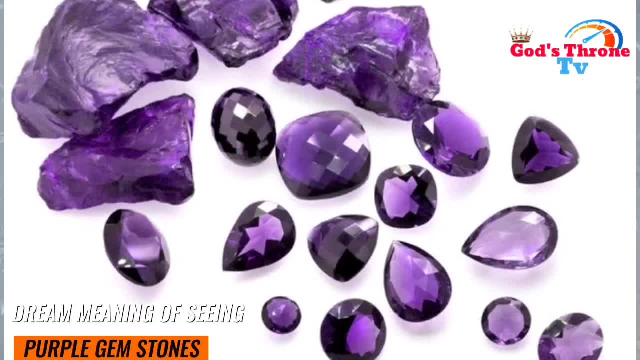 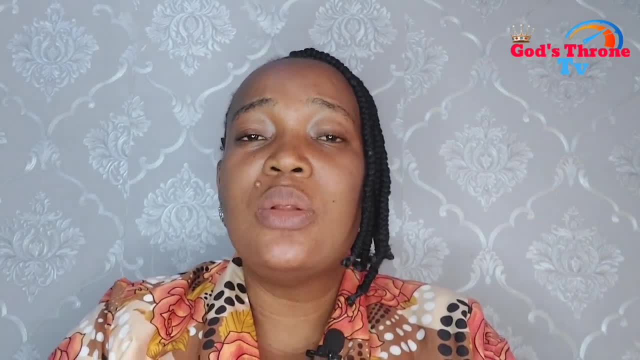 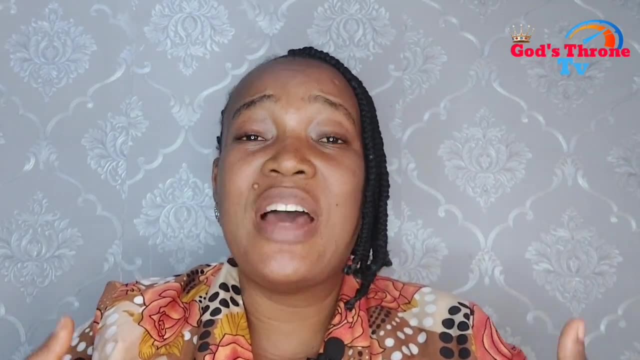 i've established the fact that purple general means generally, means authority, nobility, wealth. now, if you see, purple gemstone is trying to tell you that your office will bring you so much wealth, your office will bring you so much um, um, people will be attracted to you. okay, let me use that word. 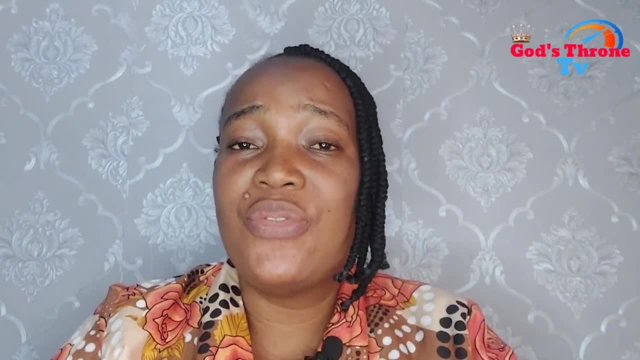 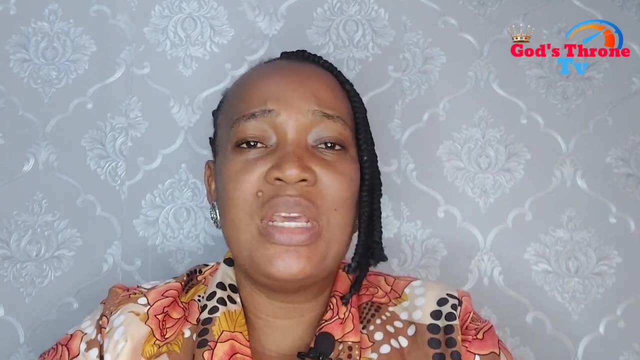 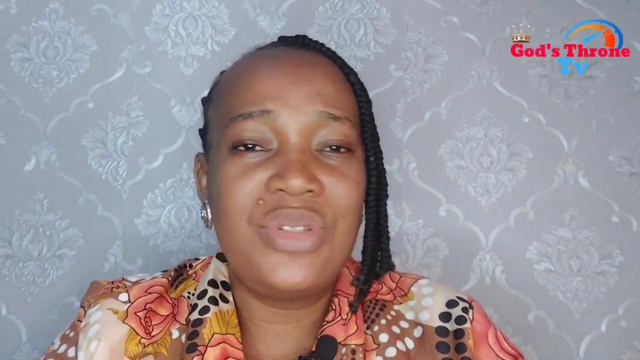 people will be attracted to you through your office, through your um, the, the, what's your, your identity? okay now, um, if you look at gemstones, generally nobody see any form of a precious stone and look away. no, nobody see a gold, silver or diamond or something and look away. people are. 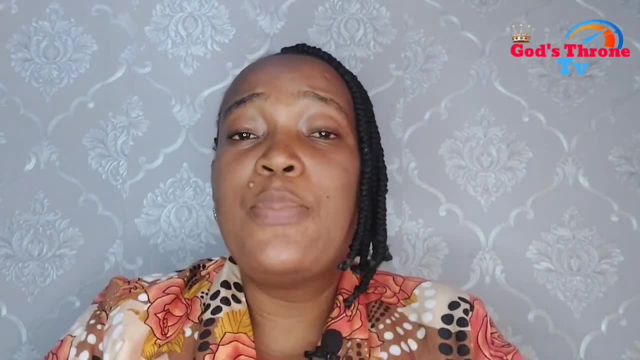 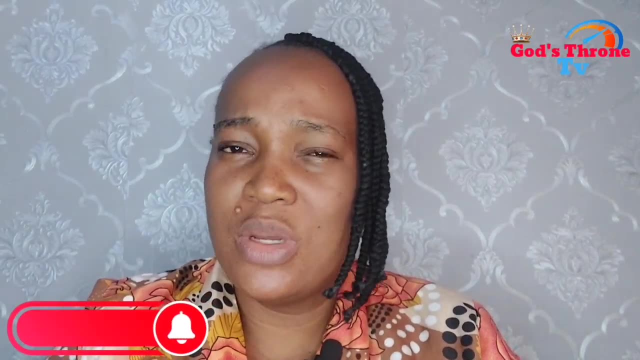 always attracted to it. people would want to touch it. people would want to touch it. people would want to touch it, want to get identified. you know people. you know in in the waking life, people can do anything just to get this gold and know. you know what, what i mean, so what i'm trying to tell you that once you 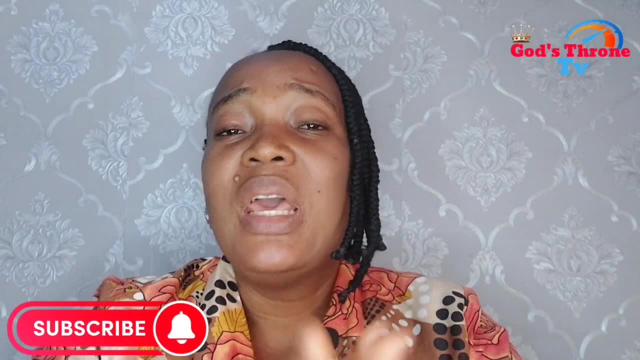 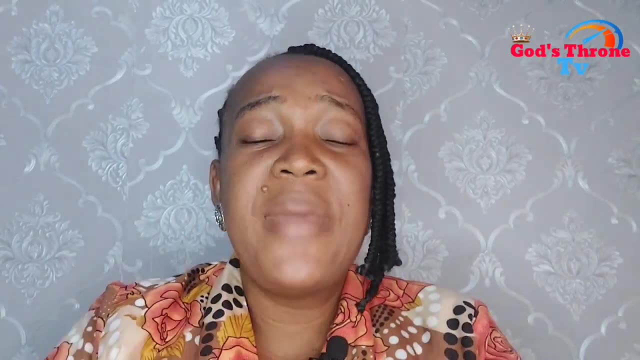 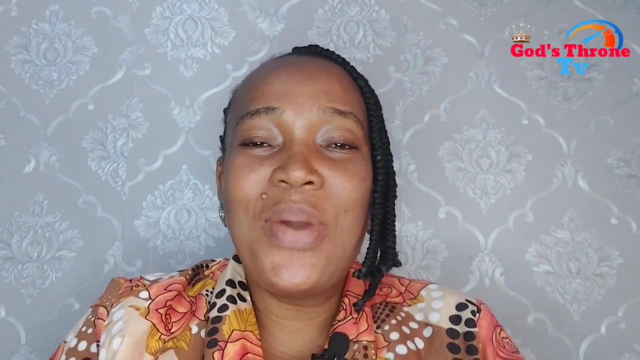 see a purple gemstone. purple gemstone it means that your office, your authority, your identity is going to attract so many people to. people would want to come, men would want to know you, men would want to just help you. okay, you know that kind of lifestyle now. you know when people 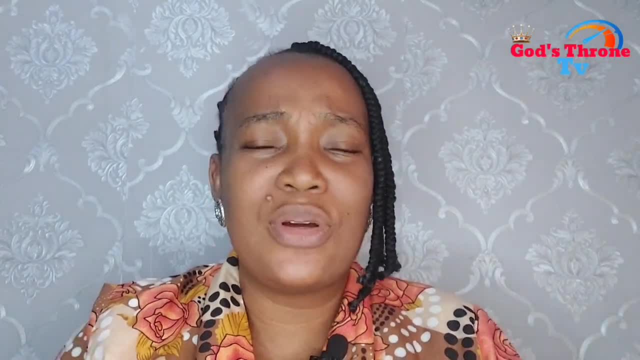 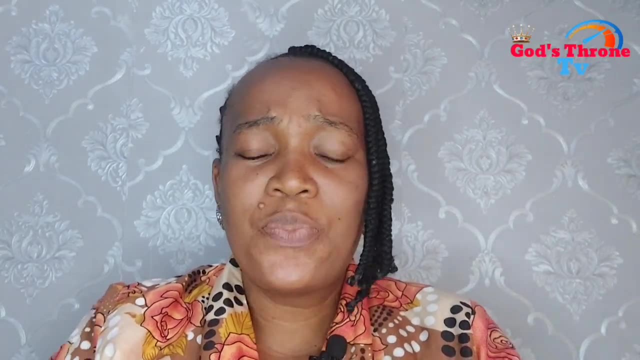 know your identity. they will just want to come across. you don't want to flock around you. they want to. they just want. they just want to be a part of you. they just want to be a part of you all right now. that is that now, when you see a flower instead of flower, that is. 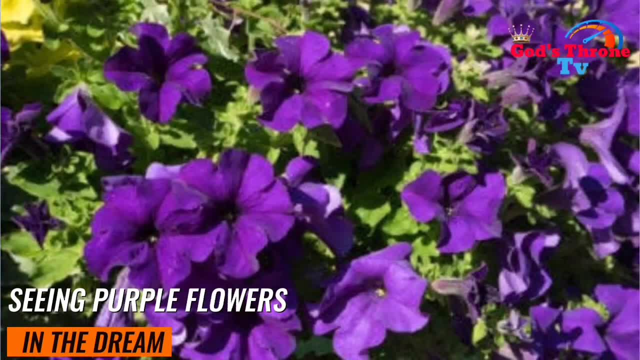 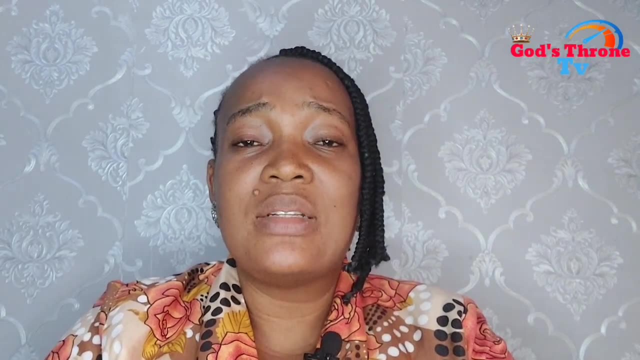 filled with most of purple now, um, a lot of colors of flowers out there, but once you see a purple flower, once you see a purple flower, like it could be, um in a flower vase or something you know, it means that, um, you need to nurture, you need to nurture. 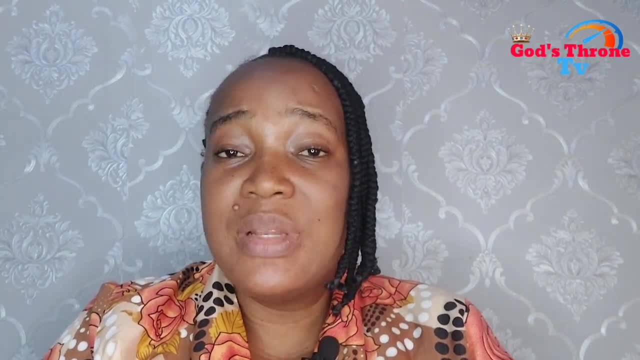 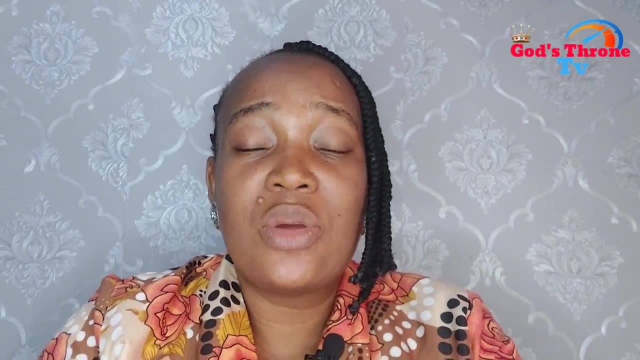 there is a seed that god has placed inside of you, which means you need to nurture it. okay, which means you're on your on your way of nurturing something very small. okay, you need to nurture it and take care of it. okay, that is what that dream is trying to tell you. so, if you have, 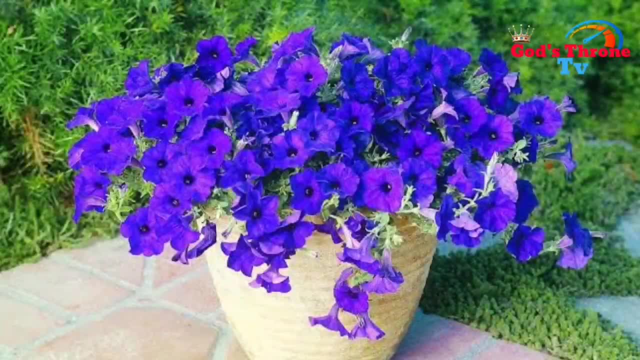 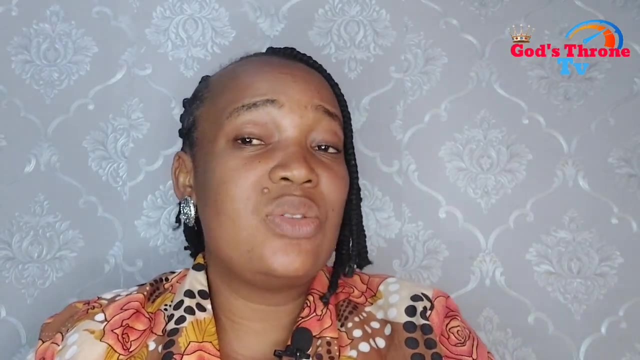 had that dream in the past. you have a flower vase that has a feel of purple, majorly purple. that dream is trying to tell you that god has placed something inside of you that you must nurture and attend to all right. so you must take note of that. now another thing you must understand. i said something. 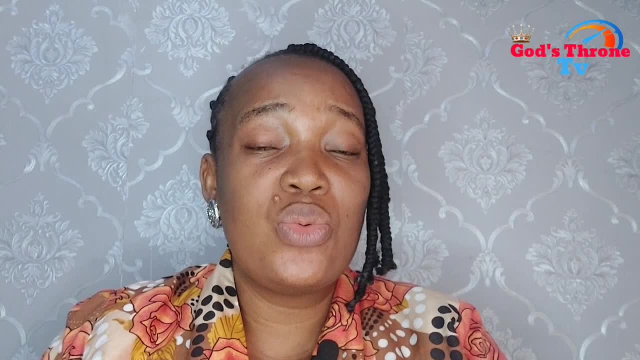 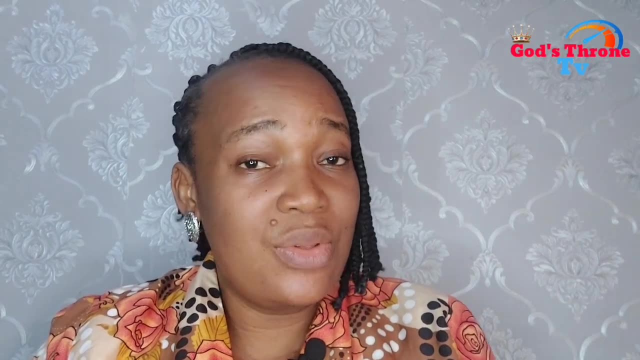 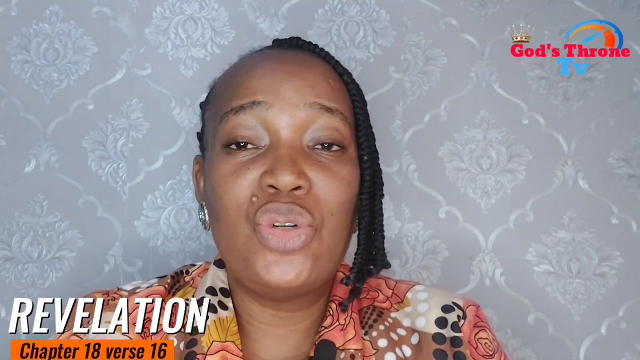 at the beginning of this video that purple color can also be, can also have um a negative meaning. okay, um, it can also. is also pointing at another aspect of your life. now in the book of revelation, chapter 18, verse 16, here now in the, god was telling john about um a particular city. now, if you um, 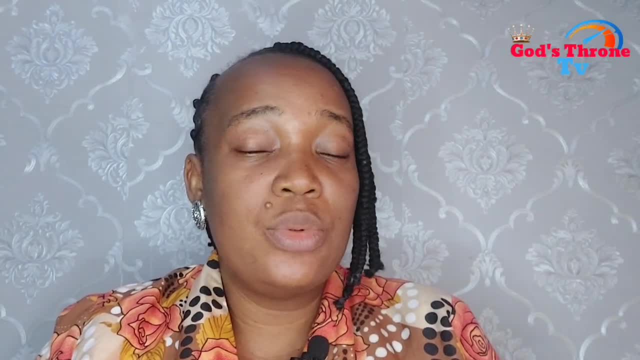 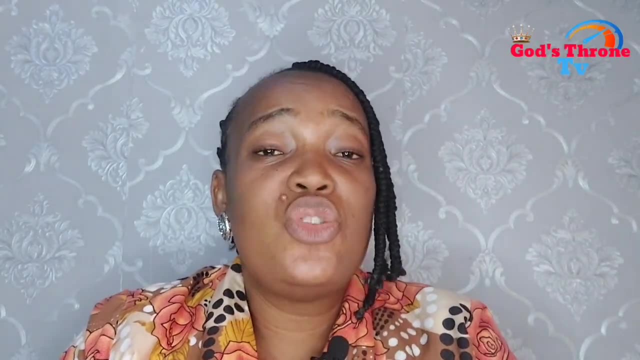 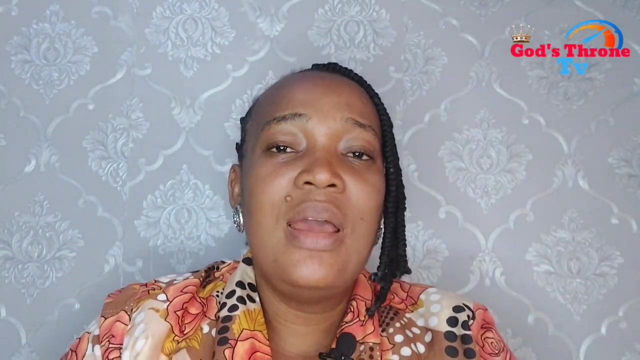 if you have a dream of wearing a purple, purple dress now, it could mean another thing, all right. it could also mean that you don't have authority, because you don't have god's authority in your life and some things are trampling on your personality- all right, which means you are not supposed to be where you are, okay. 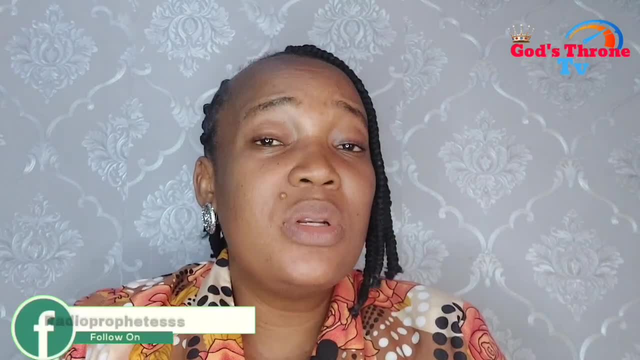 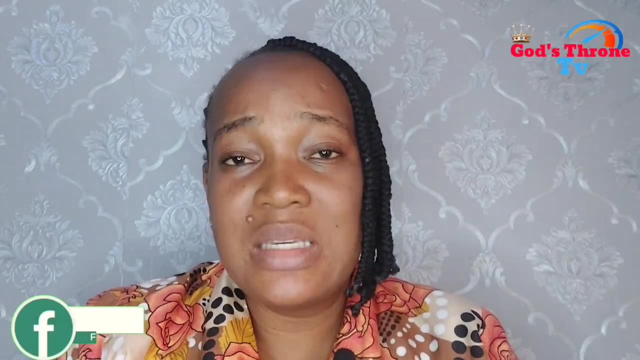 which means, um, you are not taking advantage of what god has placed in your hands, all right. which means you are not ruling okay. which means you are not dominating where you are presently. so there are two of two things. i pray that god will open your eyes, god will give you. 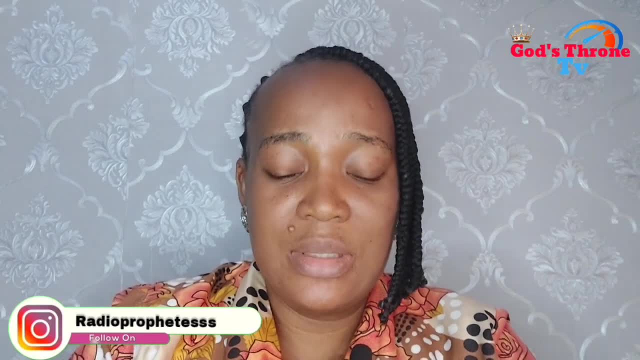 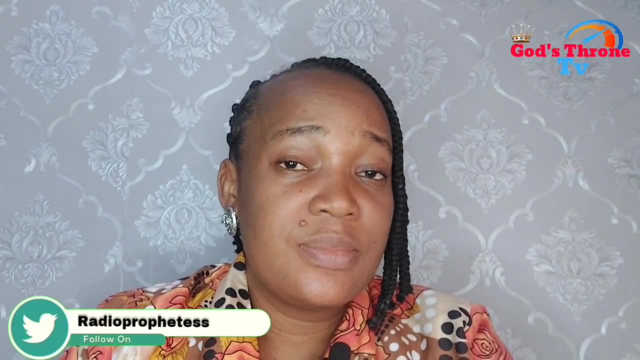 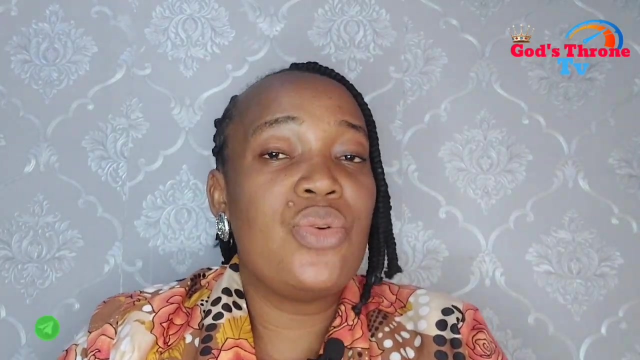 um, a great understanding of what i'm talking about this day. this could also mean that something that you are doing at that point in time is not even your job. okay, all right, which means it's not even your job also means that you need to gain more experience. okay, you need to grow now. if you look, 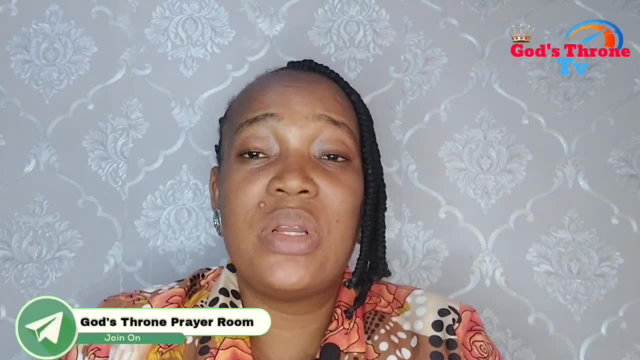 over the internet to the lot of people that not have not even waited, in this, in the secret place for god to help them grow, and they are just not in the right place. but in grace that means god is not willing soup, so their topic: unfortunately, he does not believe you, while you Obviously 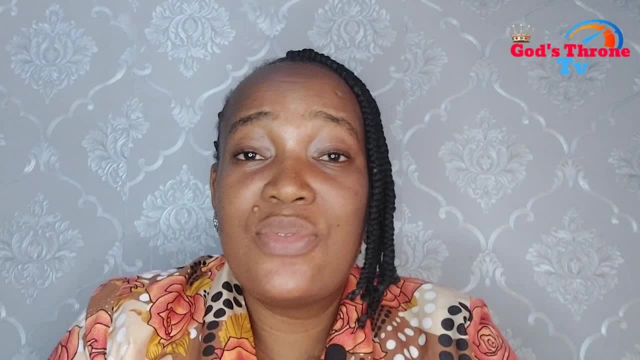 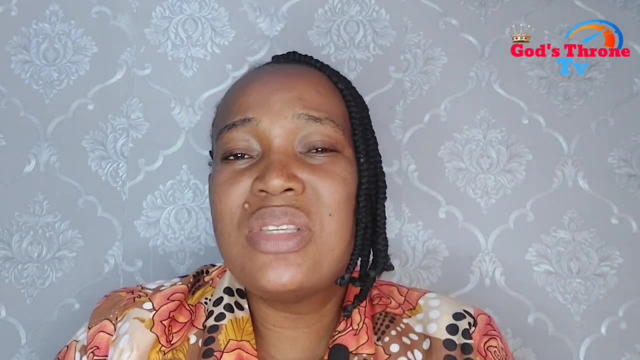 them trying to mentor people, meanwhile they themselves they are not even being mentored. okay now, which means god is trying to tell you that you need to still prepare and work on yourself. which means you need still need to ask god to help. help you increase in a certain aspect of 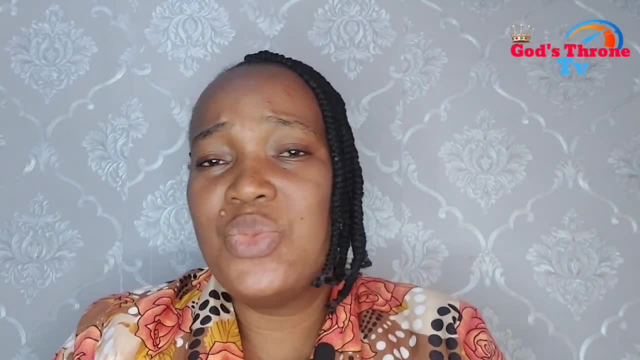 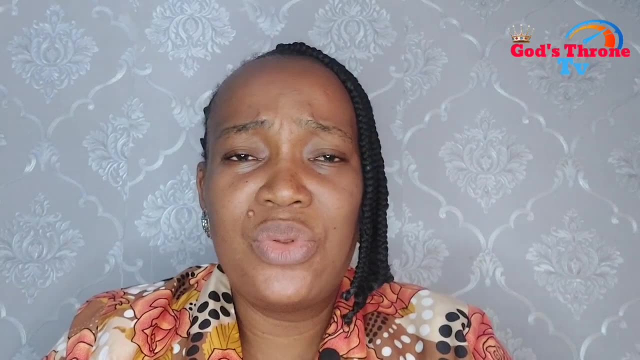 your life. i don't know whether you get what i'm trying to say, so try and relate all these things i've said to you in um with your waking life, and i pray that god will give you authority in the name of jesus. sometimes this dream could also mean that you are stepping out of line. you are not in line. 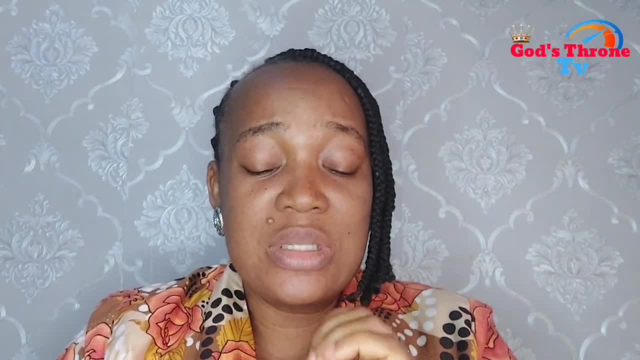 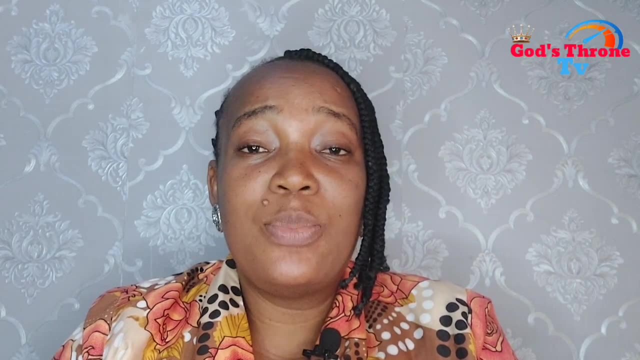 okay, you are not in line into. you know you are not in in the right direction. that god is telling you. all right when, especially when you are um the the purple dress is not even on you right now. okay, the purple dress is not on you, probably is on the floor or somewhere around you. 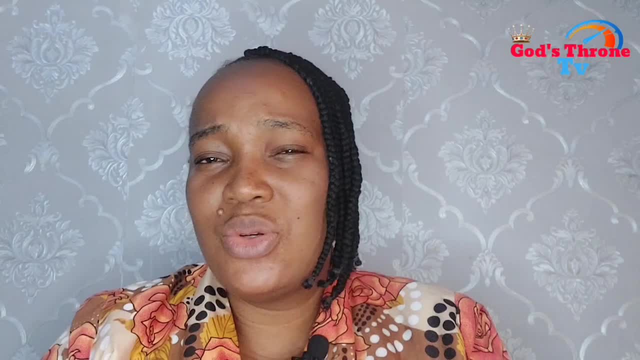 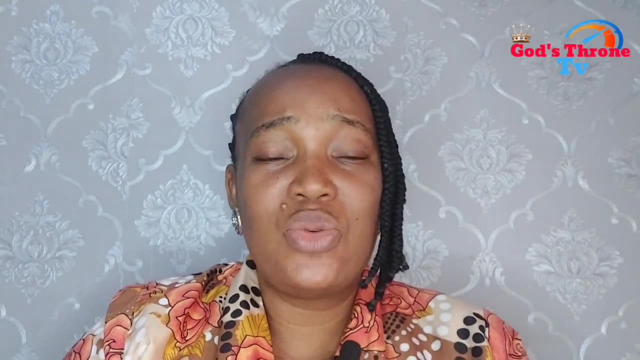 but once you see it is trying to tell you that you are not in line of what you're doing. you're not in line, you are digressing. a lot of people have lost focus in ministry today. a lot of people- not only ministry- in what god has given. 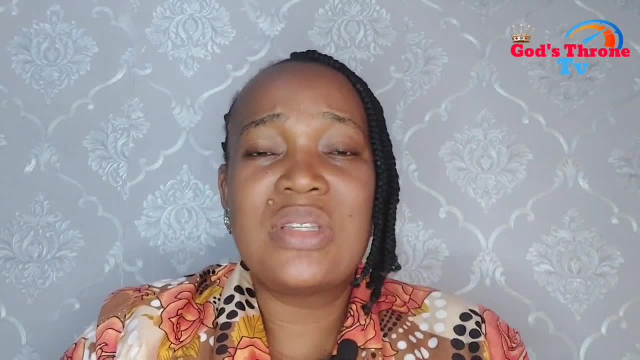 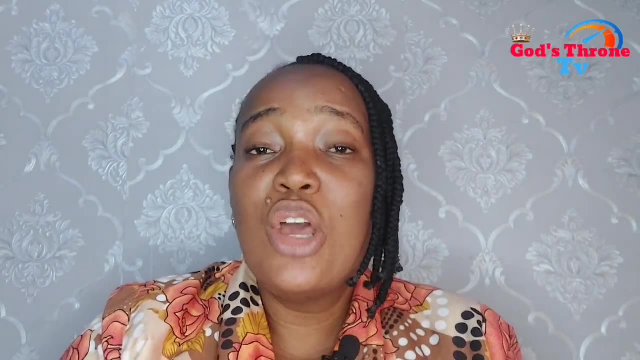 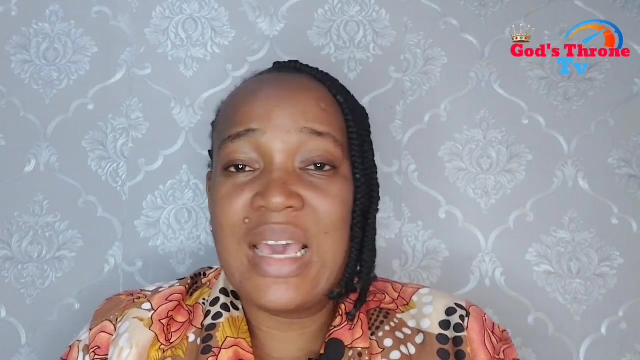 them to do. god, you know they have lost focus. they are not in the direction that they are supposed to be. so this dream is calling your attention to read that you need to make amends, you need to come back on track. okay, you need to come back on track. it's not that god's dream is not to scare anyone. it's. 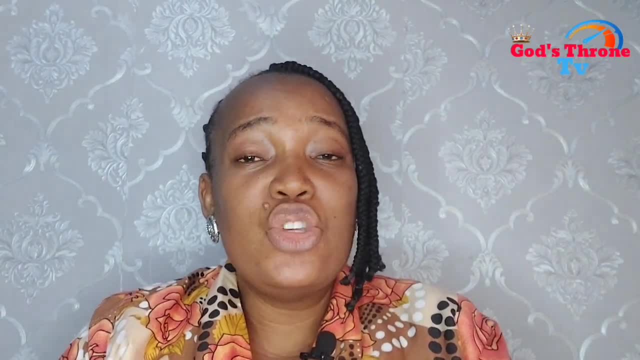 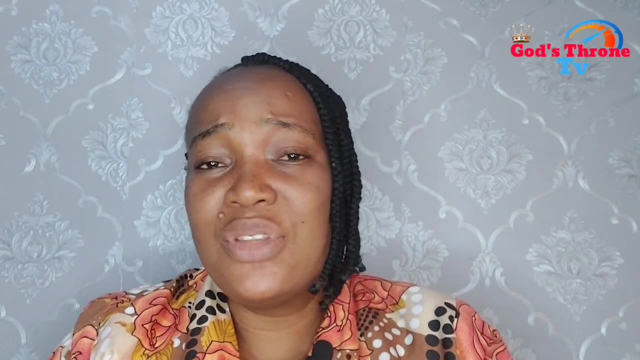 not to scare anyone, but to bring us back on track is to help give hope, is to help, you know, get those things, but it's to give you direction, all right. so if you have this dream, i don't want you to feel bad or feel scared or whatever. anyone is trying to manipulate, you know, but he's trying to tell. 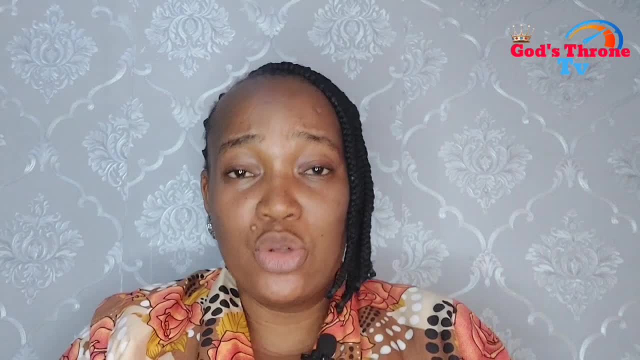 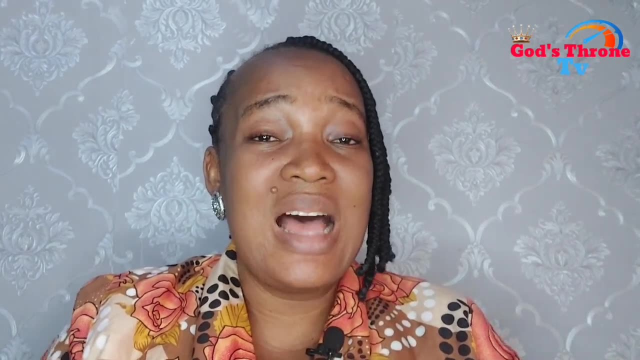 you that you need to come back? all right, you need to come back on track and make things, and make things right. ask god for proper understanding, ask god for insight, ask god that should give you the direction that he wants you to go. god does not want anyone to perish and god does not want anyone. 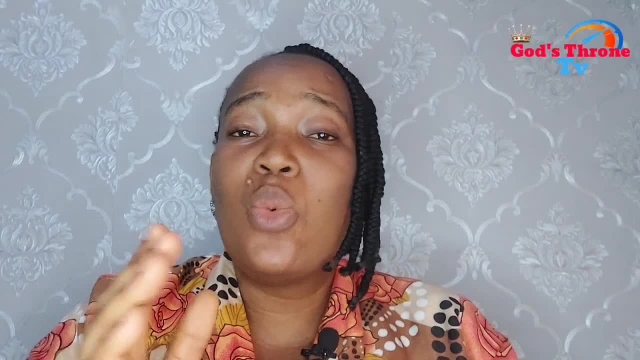 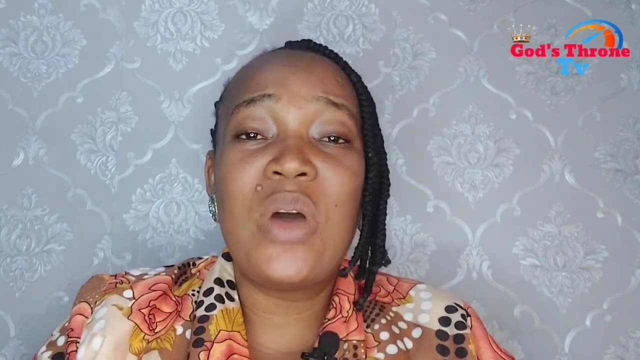 to make. the god does not want anyone to make mistake. he does not want anyone to make mistake because it's a god that is perfect, so he wants his children. he's constantly leading his children. that is why you have dreams like this, so it is not here to scare you or make you. 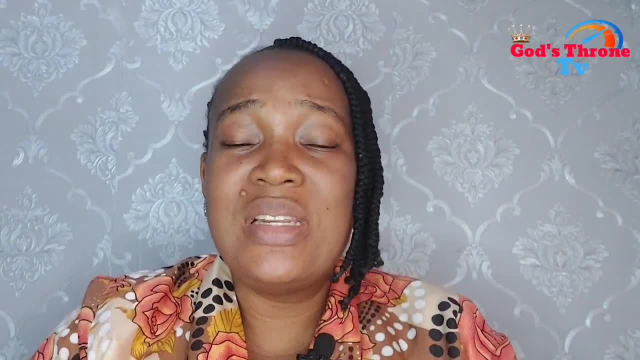 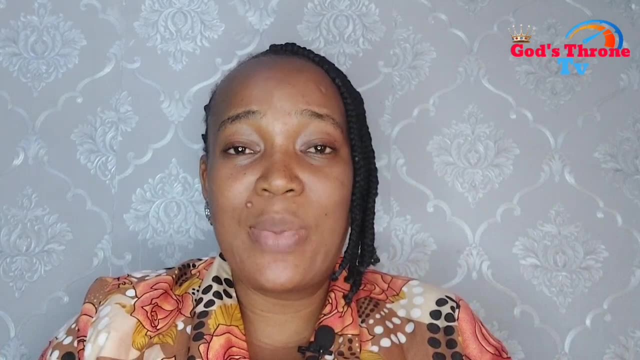 feel bad, just know that god will continually lead you and protect you in the name of jesus. now, if you have watched this video, even up to this time, i want you to like this video, because by liking this video, which means youtube would recognize this video and recommend it to.